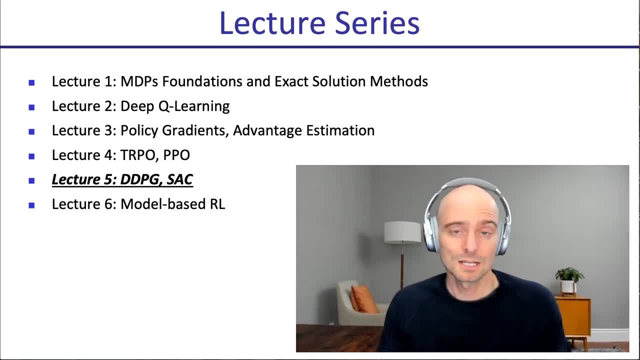 actually a lot more stable, easier to to debug, because you're always getting data from the latest best policy and this keeps monotonically- or close to monotonically if it's run well- improving over time. But the downside of these on policy methods is that they tend to be not as sample efficient. Would you care about sample? 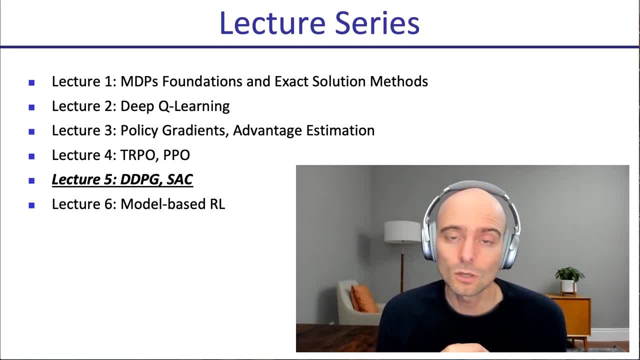 efficiency Depends on your problem. Some problems all you care about is compute efficiency and if your data can be collected really quickly because you're running in a very fast simulator, sample efficiency might not be the ball neck. Compute efficiency might be your bottleneck. But if you do care about sample efficiency, then 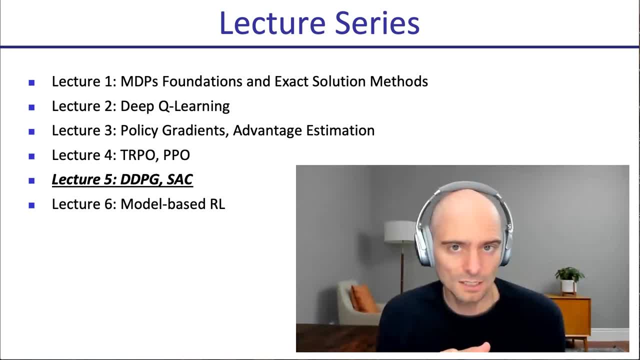 often you might have a preference for the methods we'll see in this lecture here- DDPG and SAC- over PPO, because they will reuse the data that's collected from the past more. they'll reuse it more often. so do more gradient updates per data collected, which allows the neural network to extract. 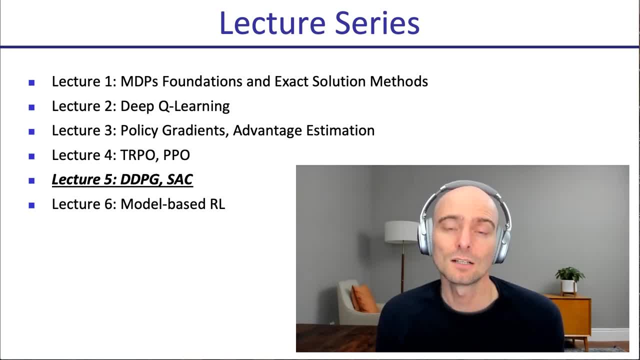 more information from the data collected and hence learn more from less data very often, And so if you look at learning curves, you'll often see like horizontal axis sample complexity, vertical axis performance, and you see that often SAC and DDPG will have a very good sample complexity, and so we'll take a look at those now. 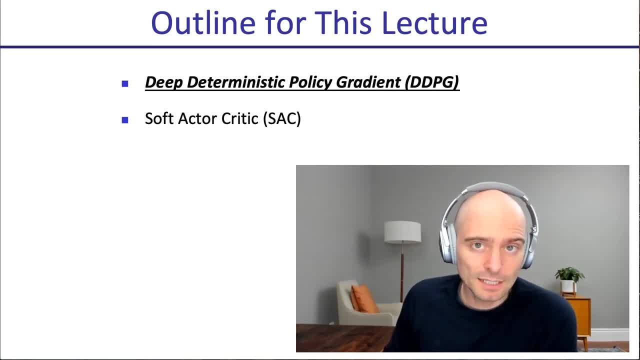 So we'll start with DDPG and then we'll go to SAC. At a high level, you can think of SAC as the maximum entropy version of DDPG. In fact, at every level, you can think of it as the maximum entropy version of DDPG. 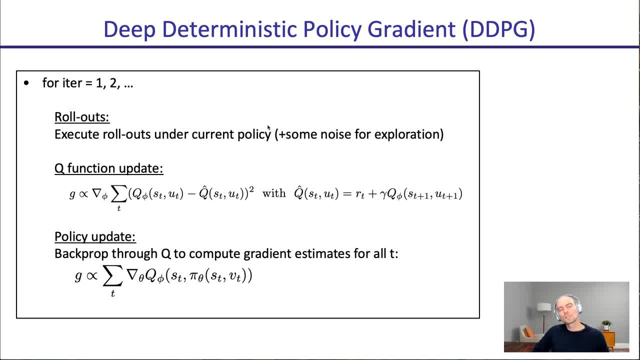 So let's start with DDPG. How does it work? You get rollouts under the current policy plus maybe some noise to make sure there's exploration. if your policy is not naturally stochastic or something, Then there's a Q function update. So, based on the rollouts, you have estimates of your Q function. 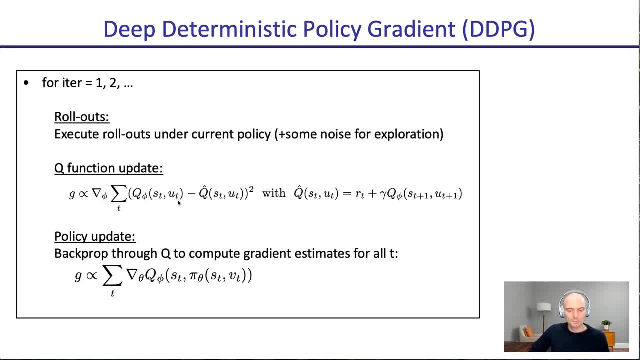 and then you do a update on this. We've seen this before. what this could be. this target here could be reward plus gamma times Q at the next state, Or you could use reward at the current transition plus reward at the next plus Q after that. 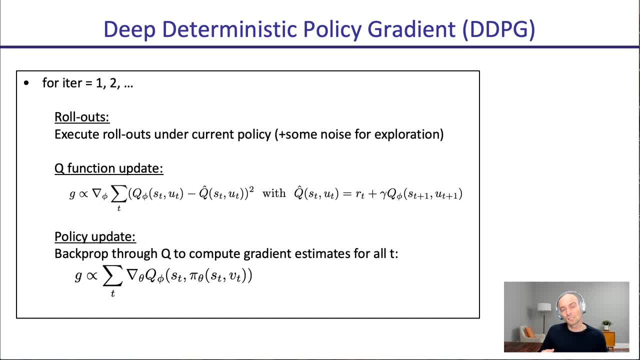 We saw this estimation. there is many variants of to which extent you take the Monte Carlo Rollout signal versus the bootstrap signal. in the original DDPG paper They use the one step bootstrap signal, but variants have been done since that are often still code DDPG where you would use multiple. steps of rewards followed by a 1 step bootstrap signal, but their events have been done since. that are often still core DDPG where you would use multiple steps of rewards followed by see the minimum momentum for SL, withInstant Q of rewards followed by a 1 step bootstrap signal, but their amout of việc. So you know, however, as long rest amout of donde you can have sumаешь your energy and the cost of 플�nt was high, but you know L. 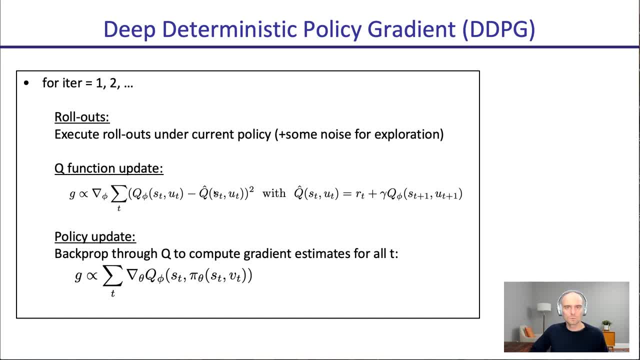 followed by the Q function as your target. So we're doing Q learning, but we're doing it based on data collected from the current policy or from a recent policy, And then we update the policy. So in regular Q learning you just keep track of a Q function. 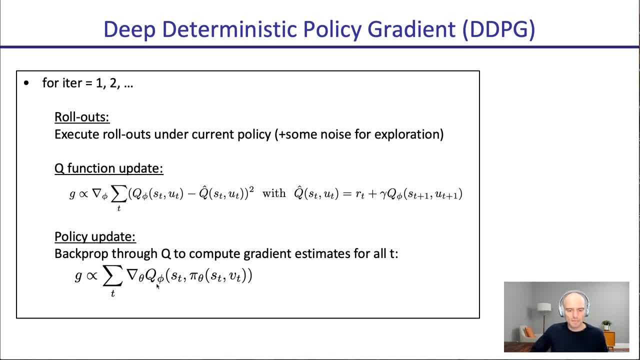 but here we also have a policy, and the policy is optimized as follows: You can look at the Q function at each state that we encountered and then there's an action we can take. This action will be chosen by the policy. We wanna optimize the policy. 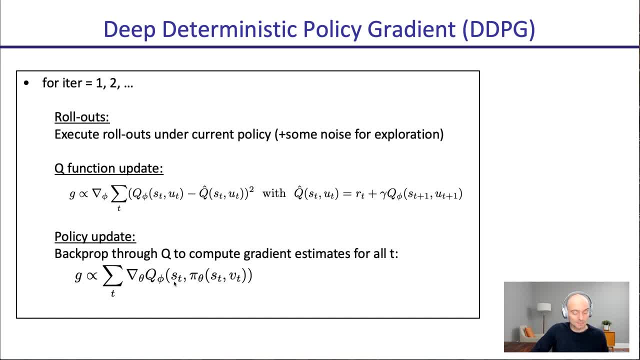 such that if we apply the policy at the states where we've collected samples, then the Q function will predict that we'll achieve a high value. So what is this saying? It's saying: optimize your policy to shift the weight or shift the actions towards actions. 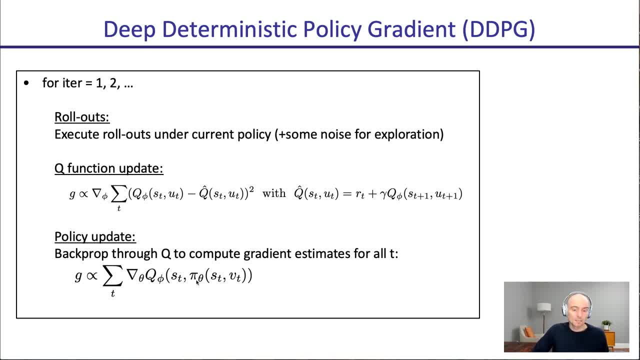 that have high Q values. And, by the way, unlike the previous policy gradient methods- the standard policy gradient as well as PPO and TRPO, which rely on the likelihood ratio policy gradient- this policy gradient here goes through the Q function. 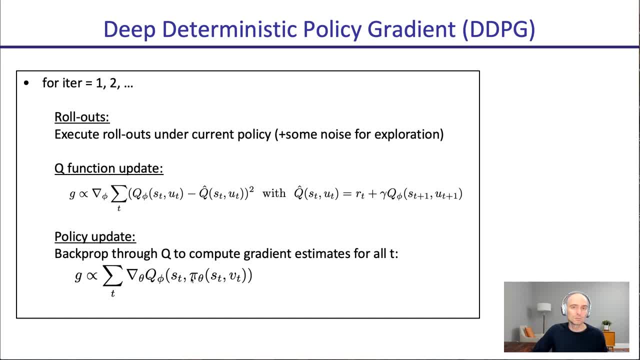 And by going through the Q function here. actually, if you want to, your policy could be a deterministic policy. Of course, for your data collection. you might still want some stochasticity and that's why it says here: maybe plus some noise. 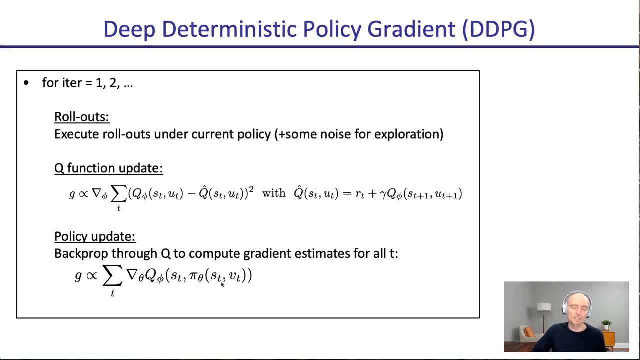 but you can have a deterministic policy. That's why it's called deep deterministic policy gradient. It doesn't have to be a deterministic policy, but it can be if you want it to be Okay, and then you repeat. So more rollouts. 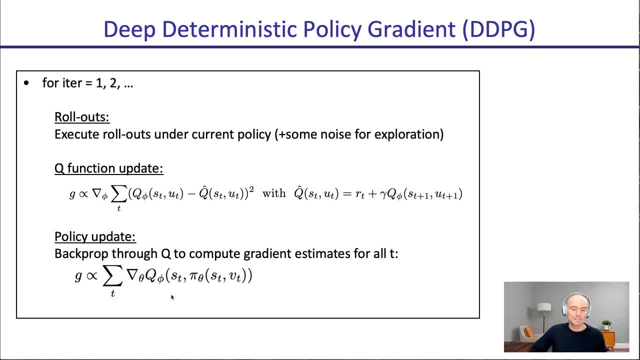 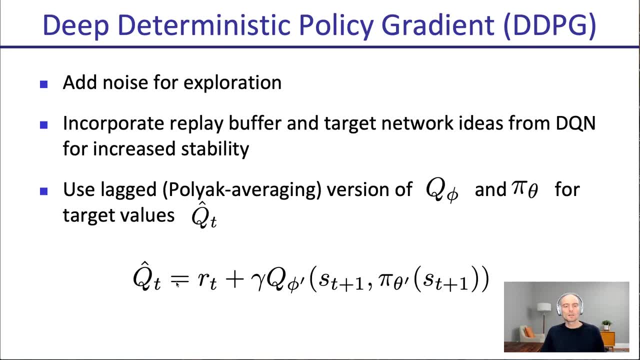 use the data to further improve your Q function estimate and then update your policy such that it maximizes Q value at the states in your replay buffer. There are a couple of extra things If, especially if your policy is deterministic, you wanna add noise to ensure there's exploration. 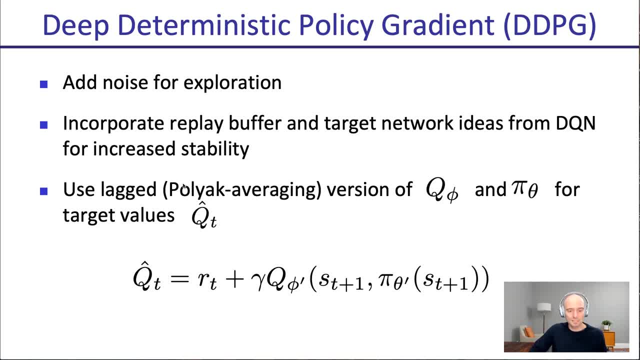 replay, buffer and target network ideas in DQN increase stability And often people use some lagged or polyhack averaging version of Q phi and pi theta for the target values of Q hat. So we have the target values You use this, just like in DQN. 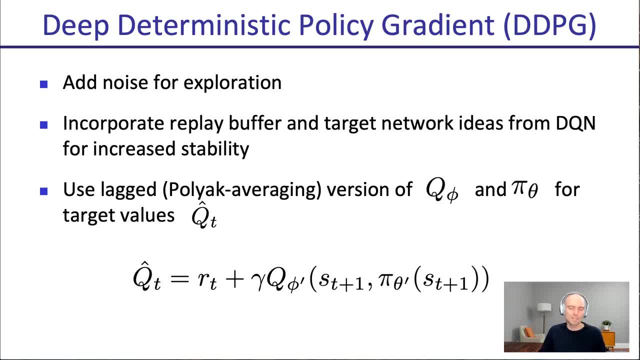 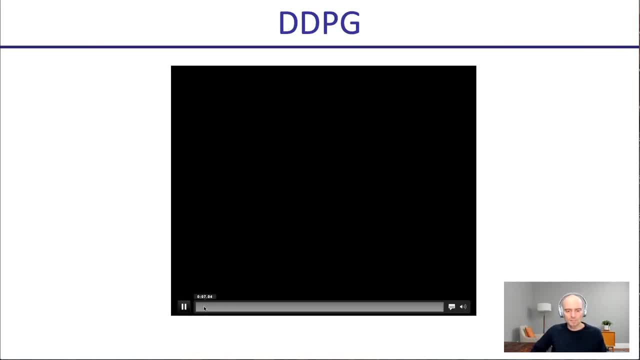 you use an older version of your Q function to stabilize things, So it doesn't like hop around too quickly. Once you do this, you can get actually really nice results, For example in simulated robotics environments. this is from the original DDPG paper. 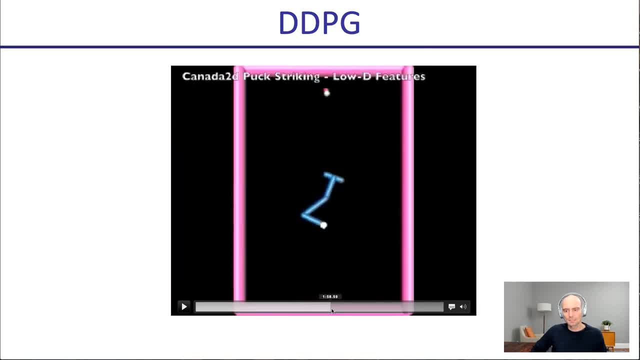 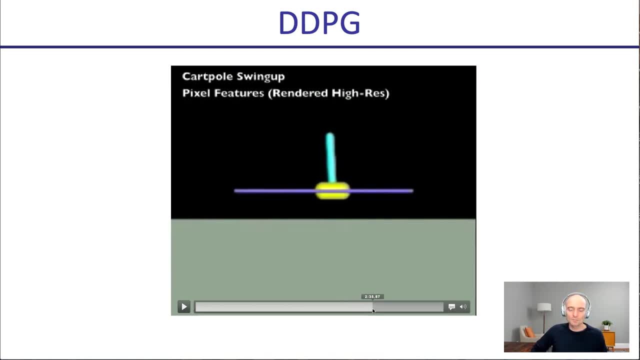 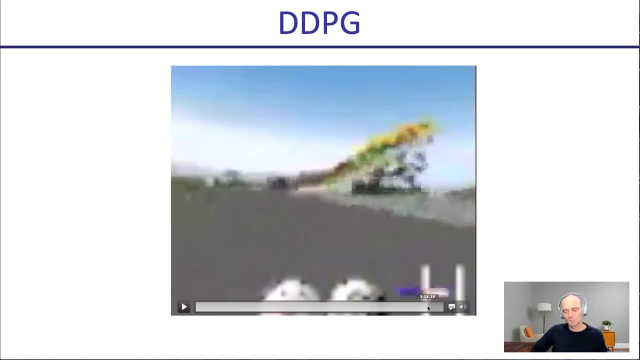 I see here a reacher, a legged robot, another reacher, a robot that knocks a ball up And so- and this is actually also done from pixels, So image input's able to learn a control policy this way. So, and even a racing game was trained this way. 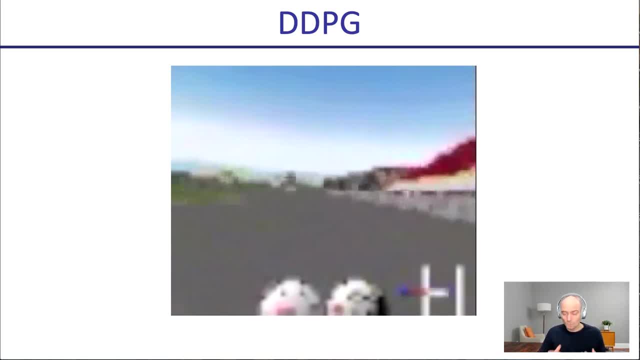 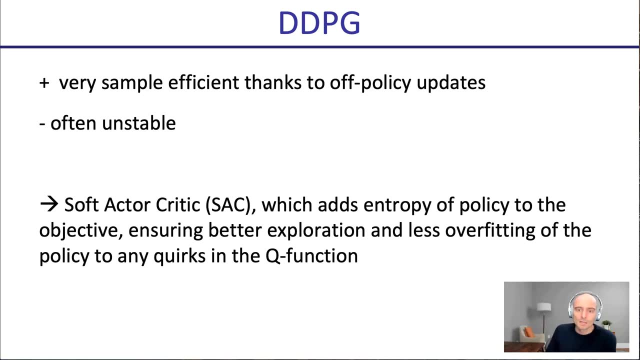 So very, very interesting that this is all possible with a policy gradient method and it'll be more data efficient than a regular policy gradient method. So it's nice, very sample efficient thanks to off policy updates. The downside of DDPG transition has been that 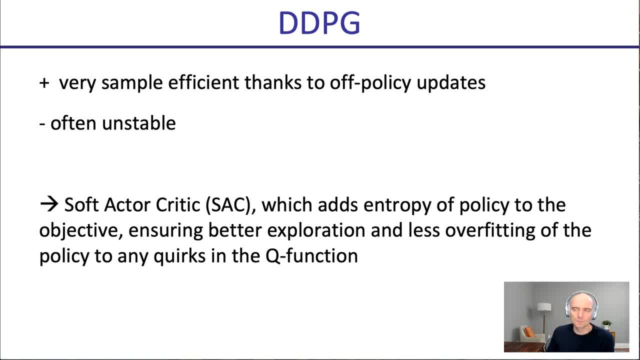 it can be a bit unstable And that's where soft tactic critic has come in and has in many places become the method of choice. It stabilizes things by adding entropy in the objective. So it's going to be a max end formulation and this will ensure a better exploration. 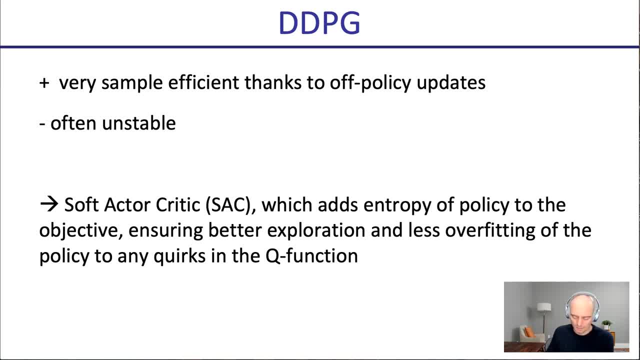 and less overfitting of the policy. Of course you need to make sure that your entropy doesn't decay too quickly, Otherwise you don't get that exploration, of course, And then the entropy, when I say less overfitting on the policy to any quirks of the Q function. 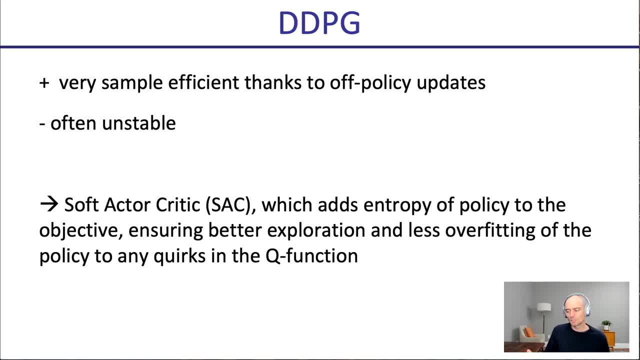 because Q function favors a specific action and DDPG might possibly heavily favor that action. but maybe the Q function is still noisy And maybe by having a max end in the objective you'll have a more spread out policy. that doesn't you know. 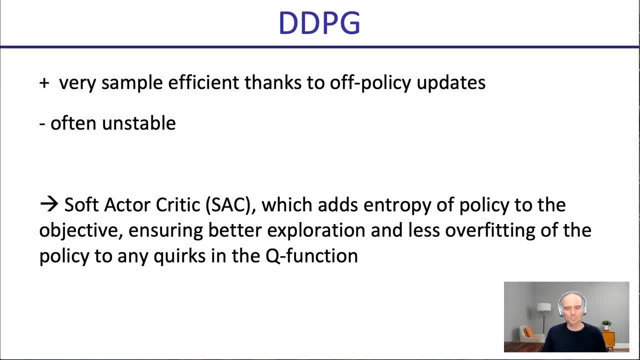 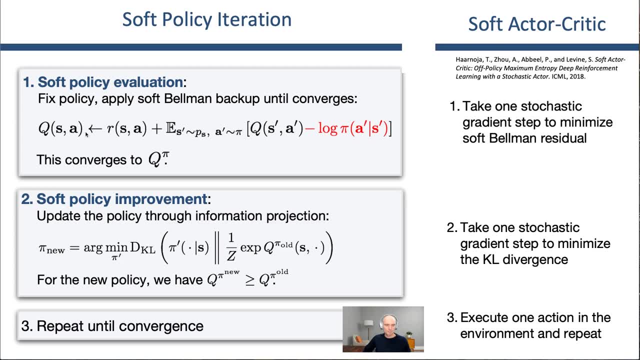 seek out to peak so highly on that specific action. the Q function currently thinks is Okay. so what does it look like? It'll use a soft policy evaluation. So if you look at a Q function, the target will be reward plus expected future rewards. 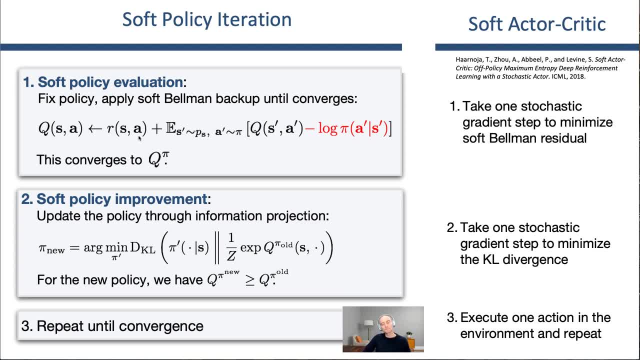 Summarizing the Q function. this first part here is a standard target, but then there will be an additional entropy term. here that naturally pops up, as we saw in the first lecture, When you look at maximum entropy. reinforcement learning: we have a reward in the objective plus. 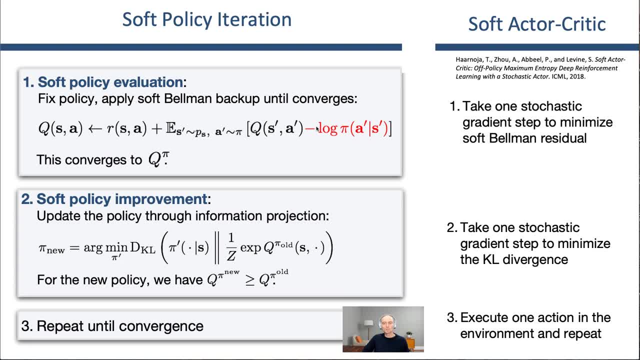 beta times, entropy. Here, beta is one. That's why there is no factor in front. Your Q targets are now adjusted to also account for the max end, Then updating the policy through information projection, meaning when you again do the thing like we saw in DDPG. 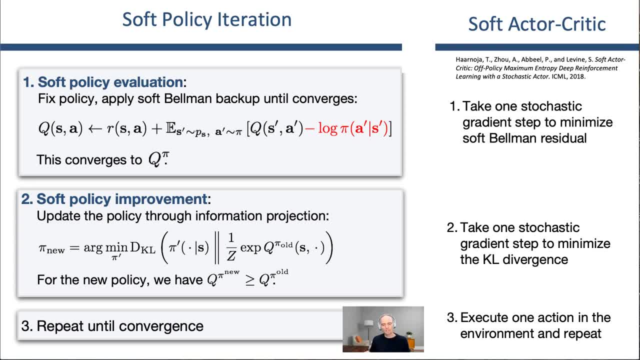 optimize your policy to maximize your Q value, You have to account for the fact that you actually now want max end policy to optimize this Q value, which we know means a policy that is effectively the exponentiated Q values. And so it's done by saying: 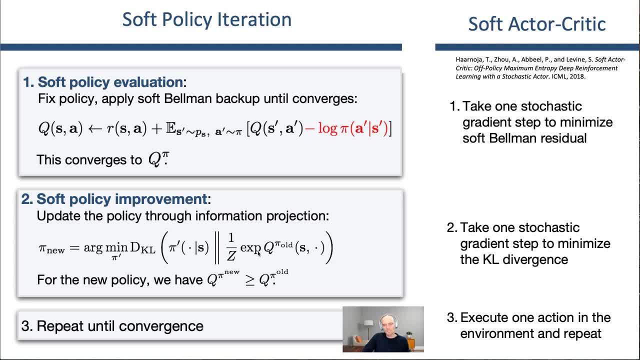 we're gonna minimize the KL divergence between the policy and the exponentiated Q values and coded policy on our samples and repeat until convergence In soft-tactile critic. of course these things are not exactly optimized, It's a iterative optimization. We'll take one gradient step or a couple gradient steps here. 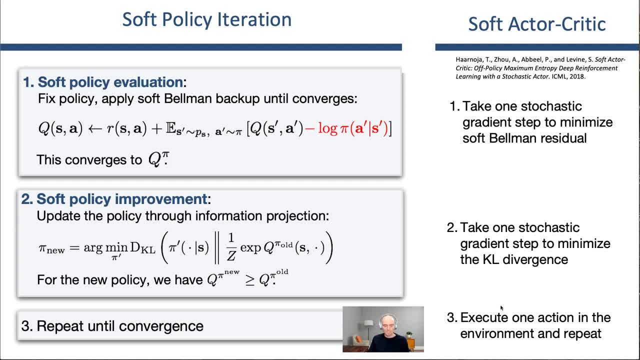 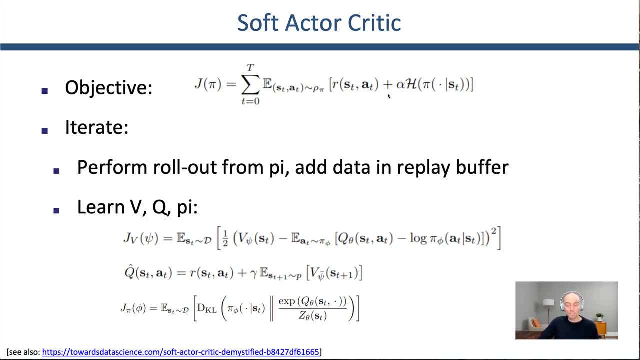 Again here on this KL objective: just a few gradient steps And then, of course, we keep repeating. So what does this look like as a whole? Our objective is now the max end objective. So if you wanna keep track, how well is my agent doing? 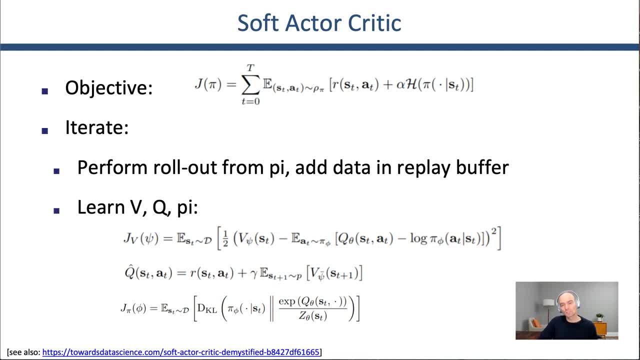 You don't wanna just plot reward. if you wanna know what your optimization is succeeding- though, you might care about reward. mostly If you wanna know what your optimization is doing, what it's expected to be doing, you wanna plot rewards plus entropy And then iterate. 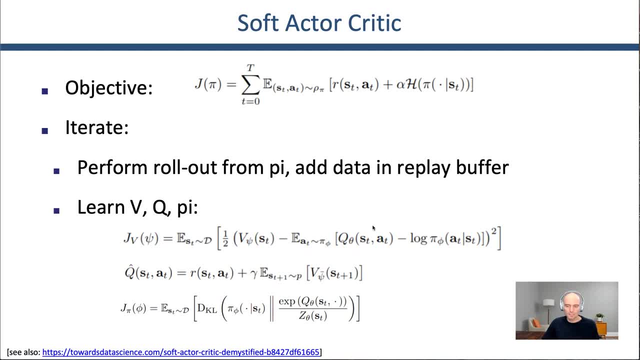 The value function estimate is this thing: here The value target is based on Q and entropy is introducing the entropy Here through the value function neural network. Then the new Q target is reward plus expected value at the next time And then the policy is based on the KL. 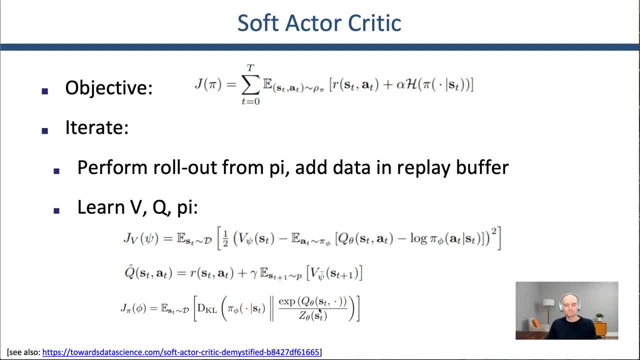 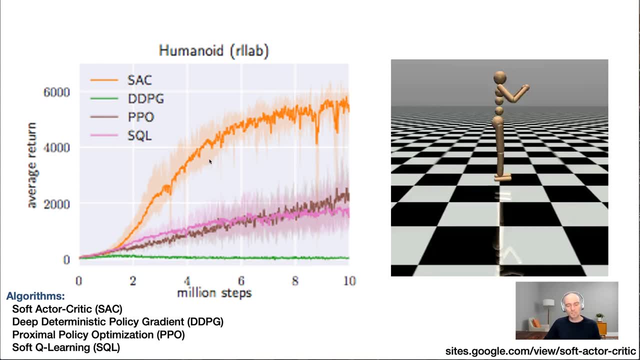 to the policy defined by exponentiated Q values. Okay, once you do this, here are some learning curves for humanoid, one of the harder simulated control problems- And we see soft-tactile critic doing really well- DDPG is here. 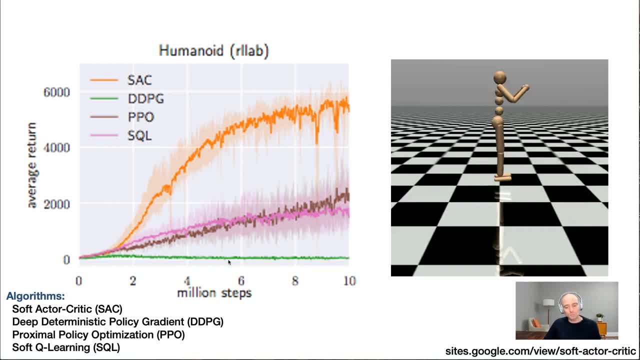 What does that mean? It probably means that either its exploration wasn't very good or when it had some good exploration, it wasn't able to extract the signal from it. With more tweaking, probably, you can make this do better. But the beauty here. 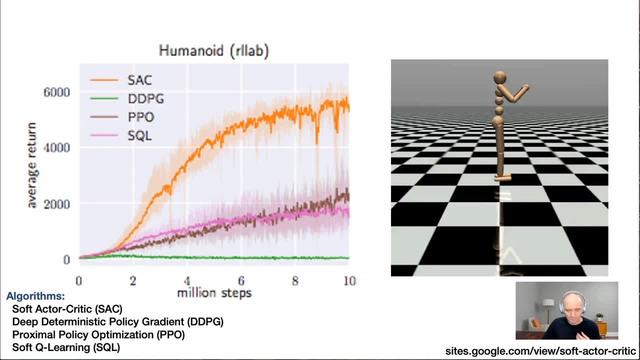 when you read a soft-tactile critic paper, which actually I'm one of the authors of, is that it's not so sensitive to the hyperparameter settings and it consistently tends to work quite well, Even across multiple runs. you can often see that even the worst run does very well. 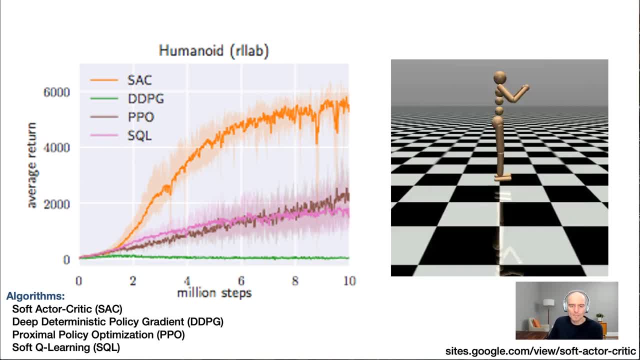 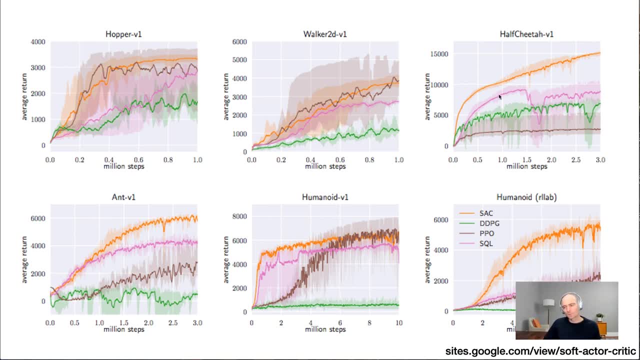 which is a really nice property. Then here are a few other environments, again in yellow: Soft-tactile, critic, consistently having really strong learning curves compared to the other methods, And that's also why it has become very often a method of choice. 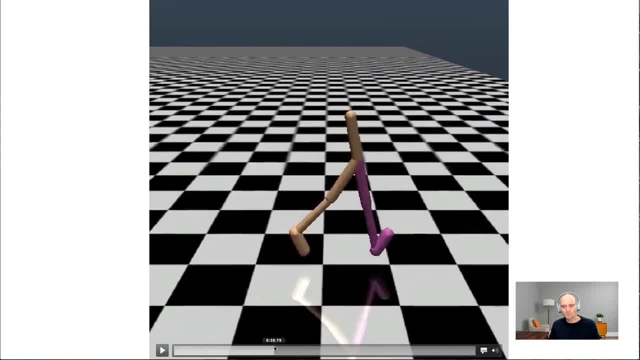 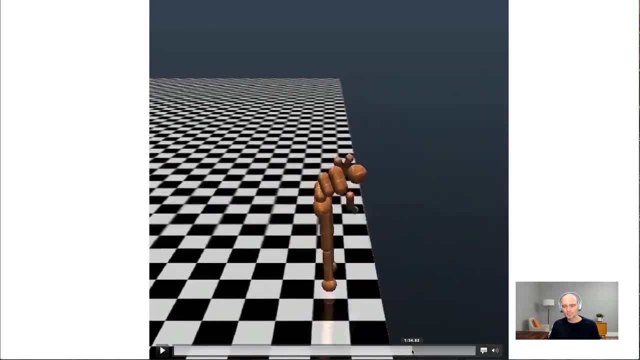 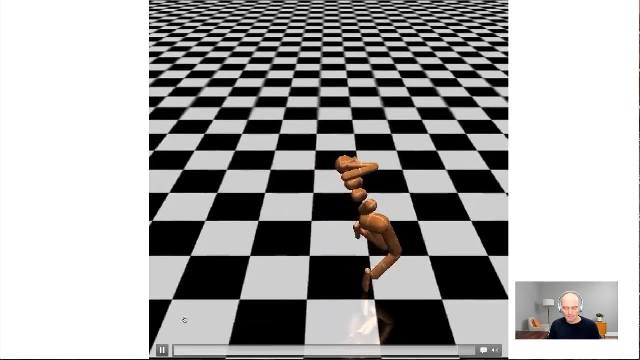 Here's the video. So hopper learns to hop really well. Walker learns to run, Cheetah runs off the grid, Ant runs off the grid, Humanoid learns to walk in some interesting ways. So what we see here is that all these canonical environments. 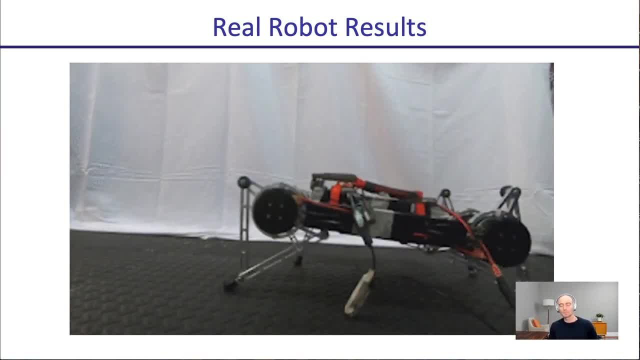 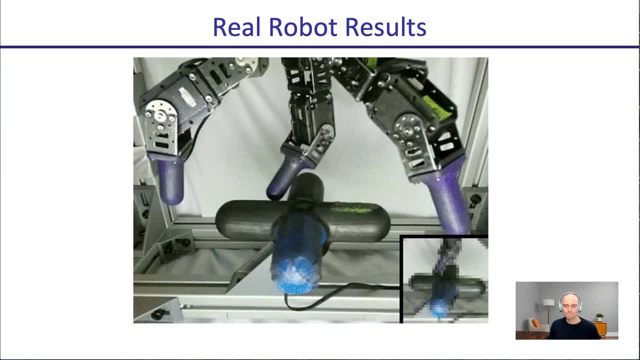 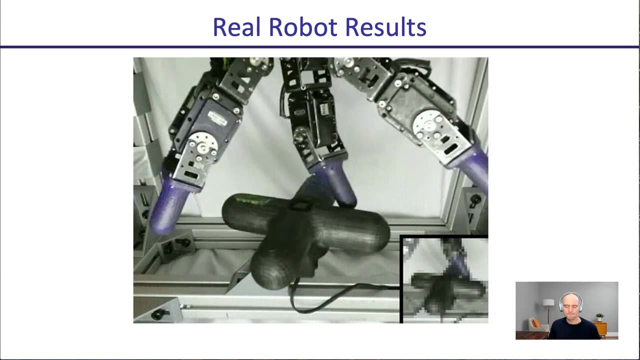 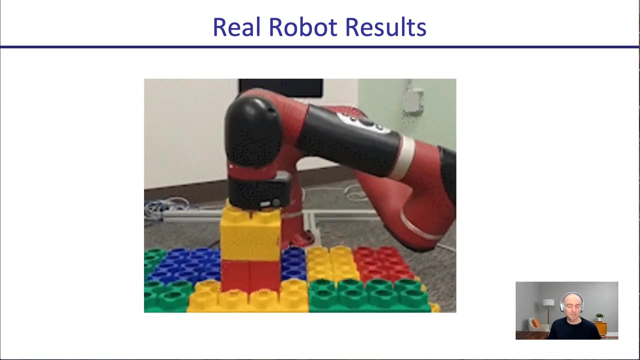 soft-tactile critic can do really well on. It's even been used to train some real robots and has robust performance there: Manipulation robots And block Lego block stacking. So it's a very efficient, robust learning method and that's why. 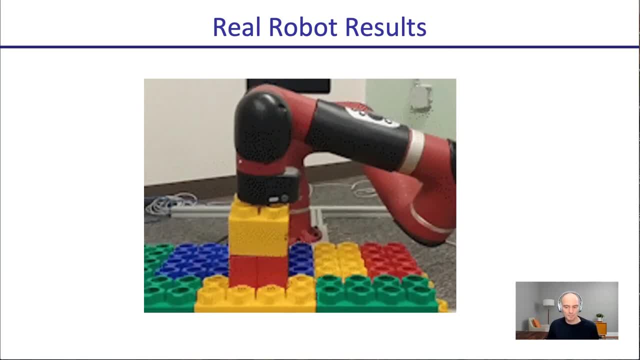 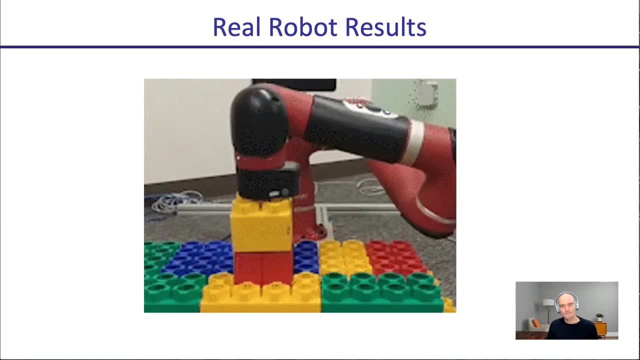 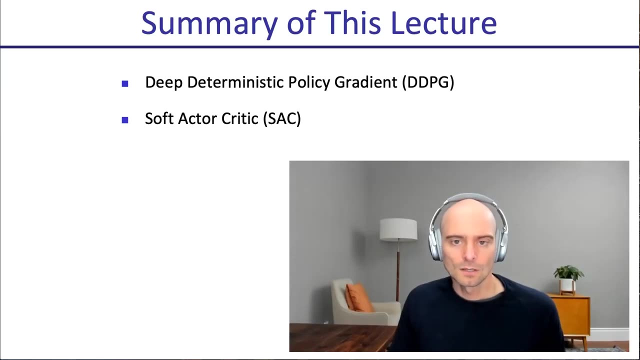 it's been amenable to running on real robots where, of course, data collection tends to be somewhat expensive and you want to be fairly data efficient to make it practical. Okay, so this was one of our shorter lectures. We covered two of the most common methods in RL today. 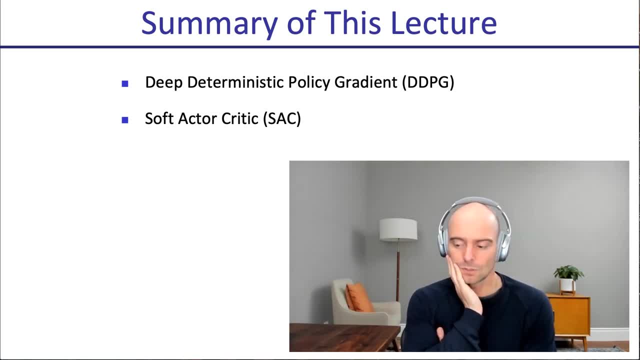 DDPG and soft-tactile critic. They compute, you know policies ultimately, but at the same time we're learning a Q function and the policy gets extracted from that Q function, And that's, in some sense, what would characterize an actor-critic method. 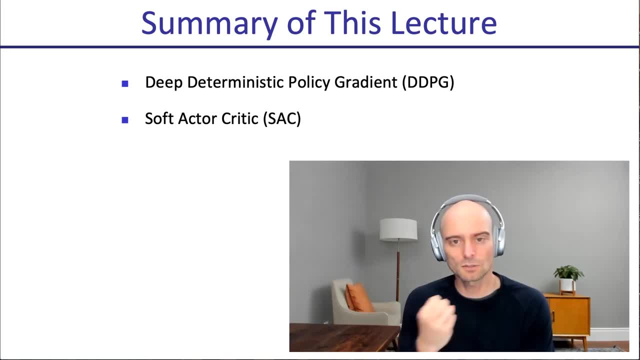 They're both actor-critic methods where the policy gets extracted fairly directly from this Q function. that's being learned.